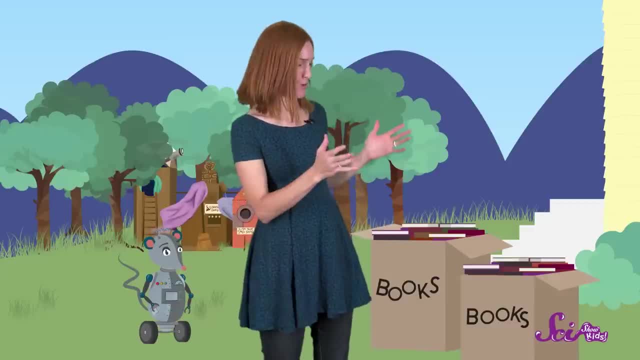 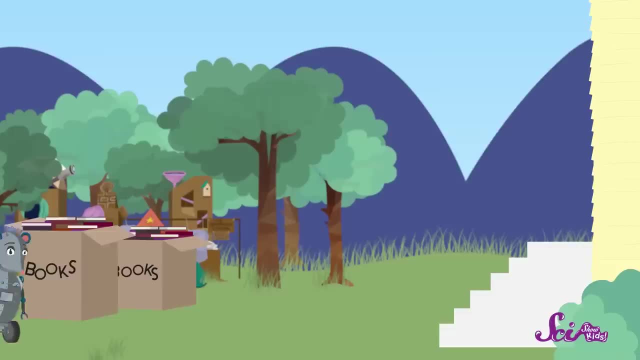 and our work is done. So let's see how a ramp can make the work of moving these books into our house a lot easier. We already said that the boxes of books were too heavy for me to carry up the steps, So Squeaks and I will put a ramp over the steps. 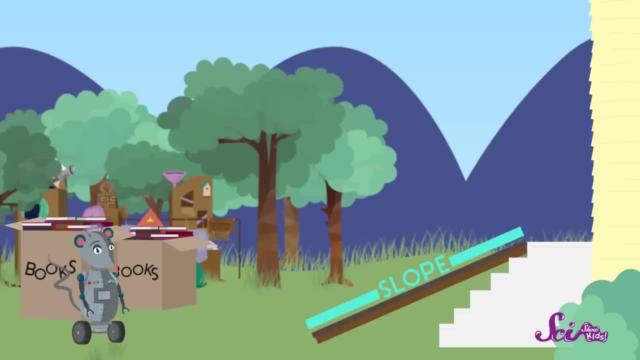 The slope of this ramp is a little steep but it reaches all the way from the bottom of the steps to the top. So if we put a box on the ramp and push, He did it. Nice job, Squeaks, Squeaks had to push really hard but he got the box to. 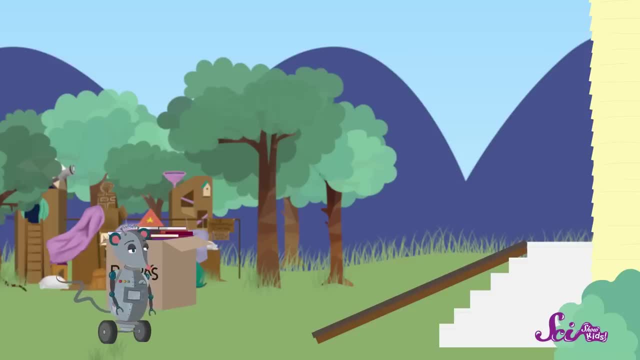 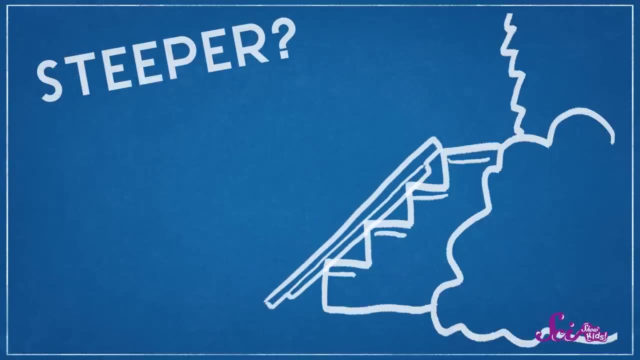 the top of the steps. What changes do you think we could make to a ramp to make Squeaks' job a little easier? Should we make the slope of the ramp steeper, or should we make it less steep? Let's try using a different ramp, one that's longer. 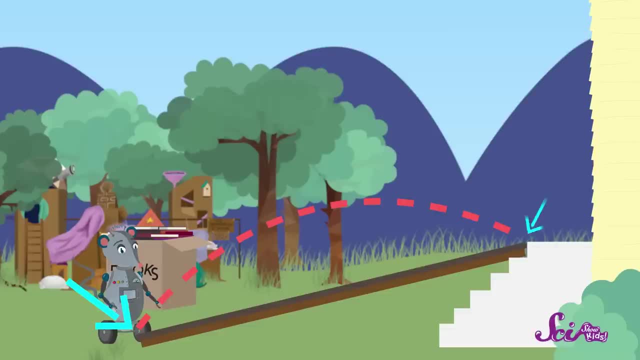 This way we can put the low end of the ramp farther away from the high end. Can you tell the difference? This ramp has less of a slope than the first one we used. Well, let's see if it helps. Ready Squeaks One, two, three, push, Yes, right up the ramp. 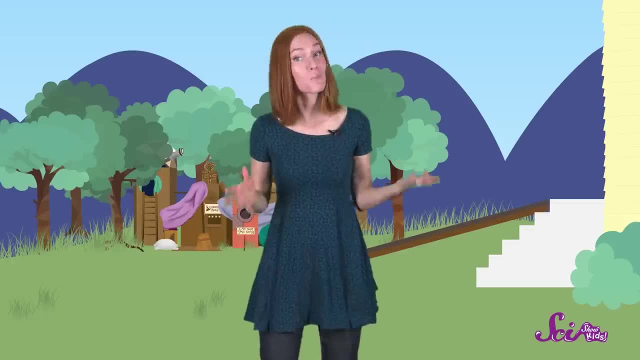 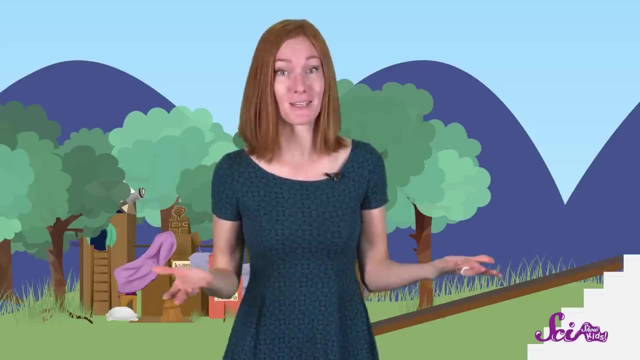 and you did it Right up the ramp and into the house. Squeaks had to push the box a little farther to get the box up the ramp, but he didn't have to push nearly as hard. When you think about it, using a ramp is kind of like walking up a big, steep hill. 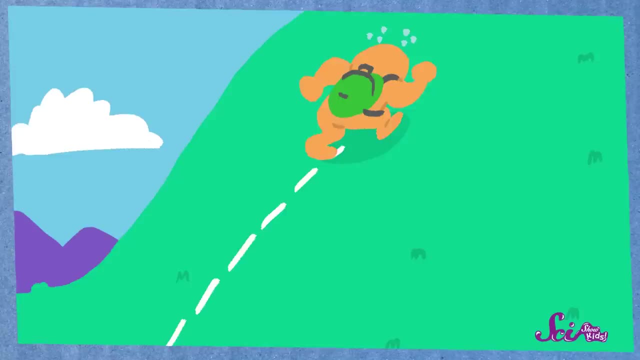 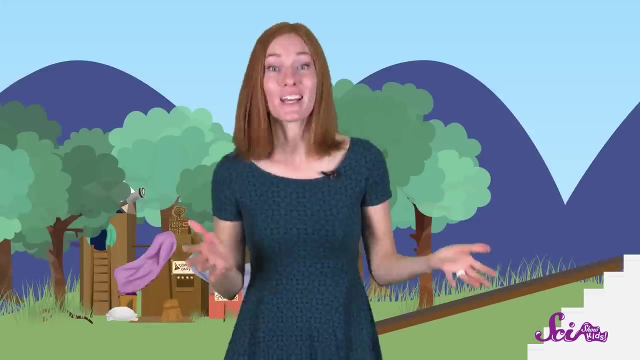 It's harder to walk up a big hill if you walk straight up, but if you take a longer path that's less steep, you'll have to walk a longer distance, but it won't be nearly as hard. In the same way, it's harder to push something up a ramp with a steep slope than one that's. 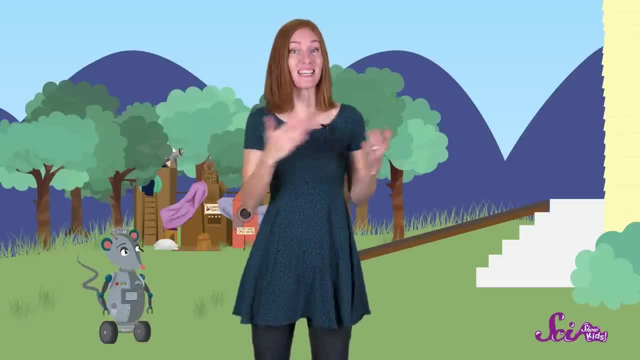 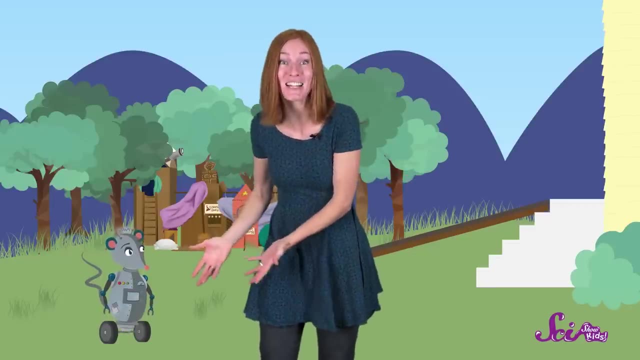 not, as steep. Ramps are all around you. They help us to move things into and out of trucks, move cars on and off of highways, and they let shopping carts, wheelchairs or robotic rats get on and off. sidewalks And ramps are only one kind of simple machine. 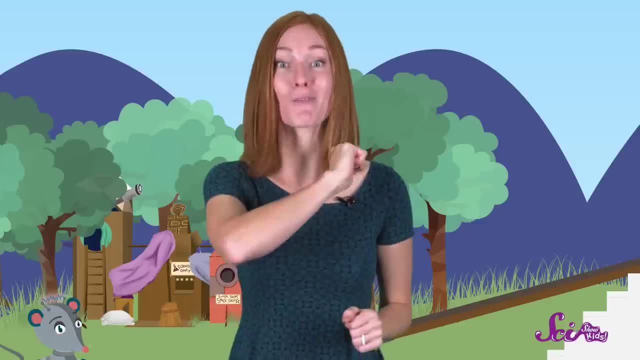 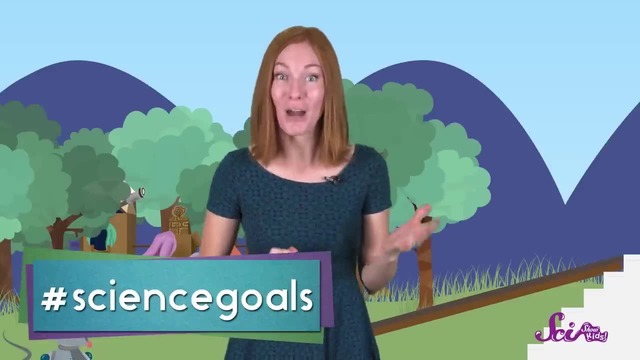 We'll explore other kinds of machines soon, but right now I'm ready to get started on one of my new books. Thanks for joining us on SciShow Kids, and I'd like to give a big thank you to Google Making Science for helping us make this episode. 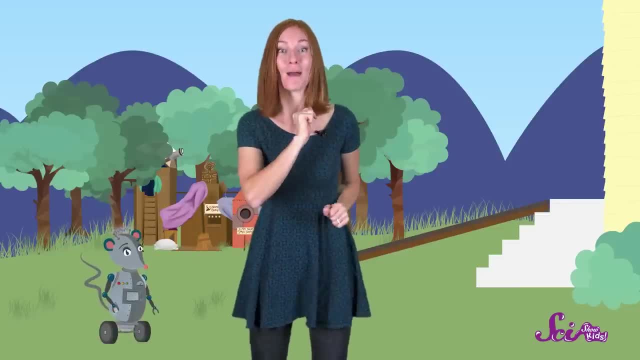 If you've got a question for Squeaks or me, ask a grown-up for help and leave a comment below, Or send us an email to kids at the SciShow dot com, and we'll see you next time.